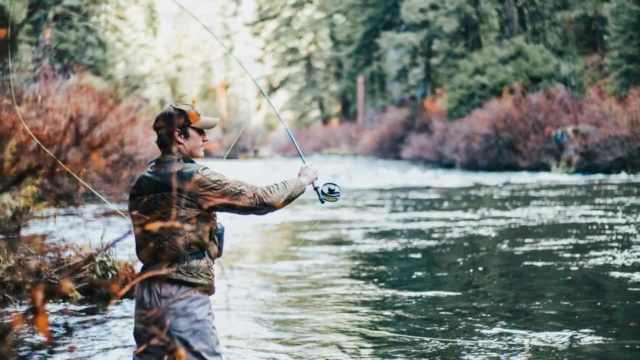 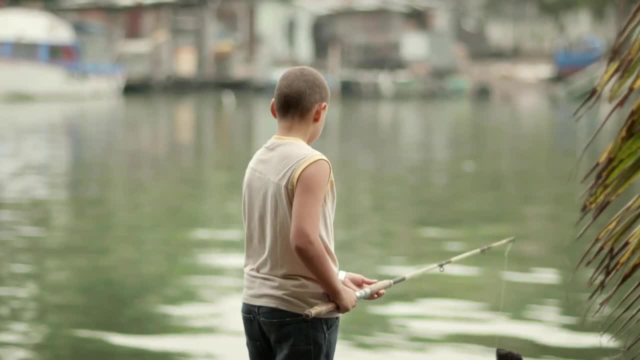 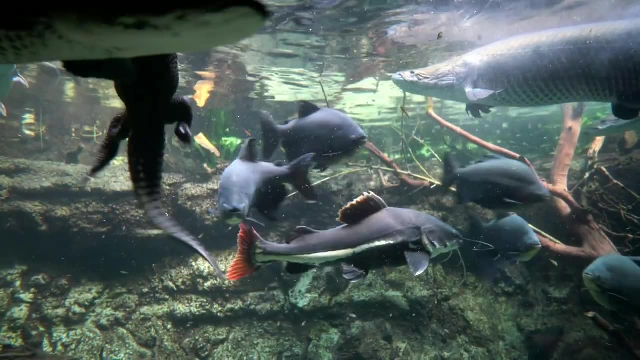 Don't get me wrong. I am not saying humans should stop fishing, but we should all follow best fishing practices and make use of equipment that does not deplete the marine ecosystem. Number 3. Water Pollution. Pollution account for the highest death toll in the marine ecosystem. 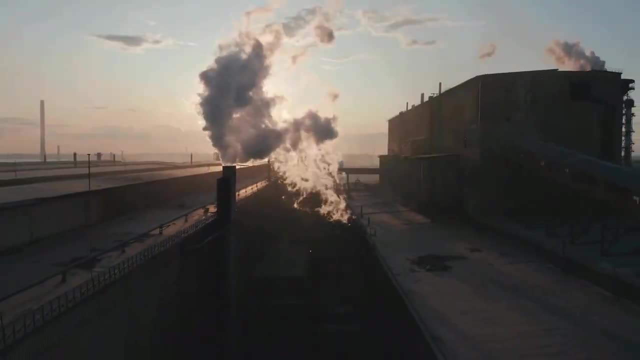 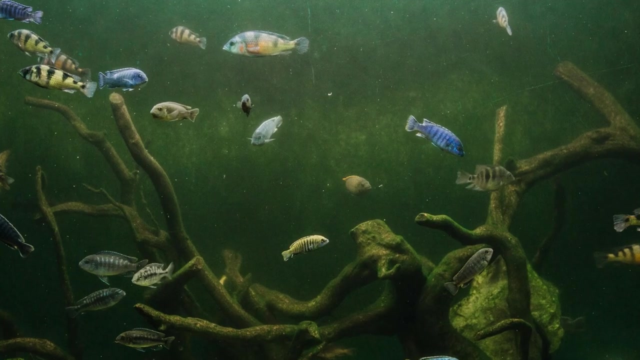 From atmospheric waste to excessive nutrient and other land source water pollution, humans have caused an untold disaster in the marine ecosystem that will take several years to fix. Being the broadest of all human activities affecting marine life, I decided to outline each and every one of them. 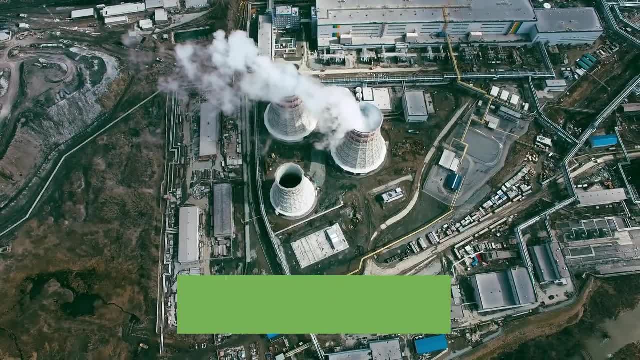 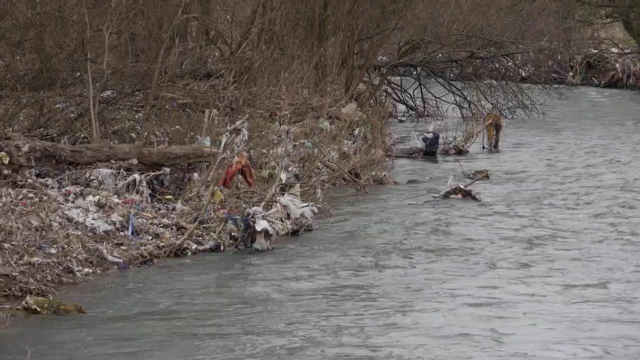 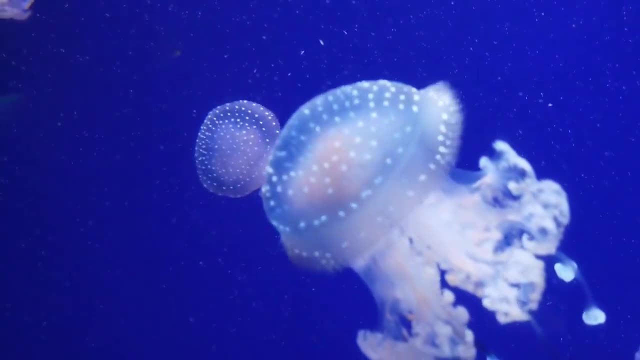 Let's look at each source of water pollution below Industrial Waste. Disposing of industrial waste, such as chemicals and hot water used for cooling industrial machines, is very common in our world today. The temperature of the water is way higher than that of the sea or ocean, thus disrupting the balance in the marine ecosystem. 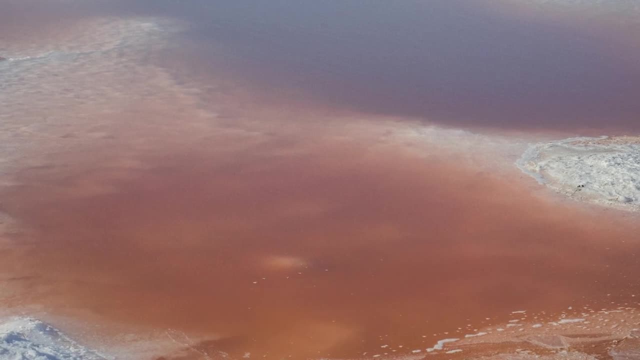 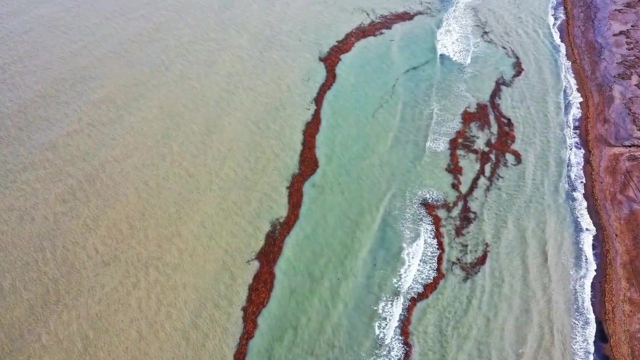 Oil Spillage. Although large-scale oil spills do not occur often, however, when it is highly disastrous, when it does, Crude oil spillage can last several years in the sea, suffocating thousands of sea creatures throughout its stay. Land Runoff. 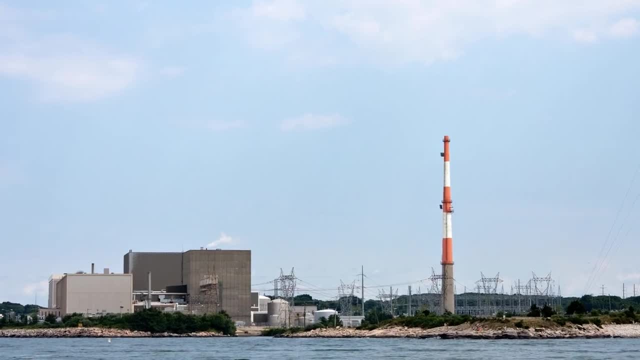 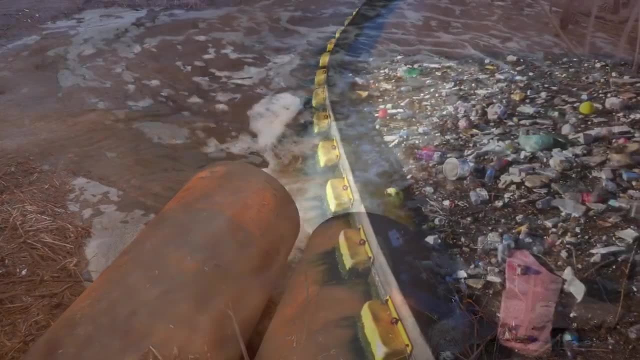 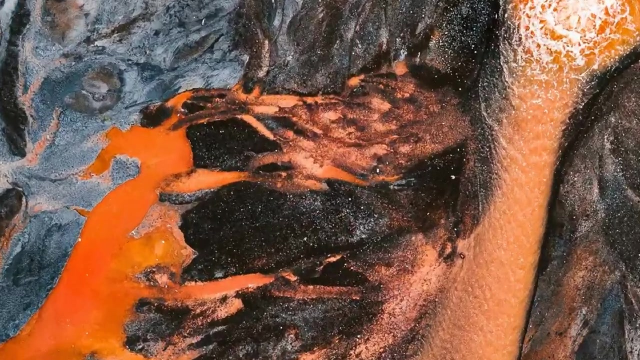 Runoff from land is one of the leading sources of water pollution. Harmful chemicals on land, especially agricultural wastes, are washed into water bodies once it rains, Therefore introducing excessive nutrients, pesticides and other noxious chemicals that are detrimental to the health of marine life. 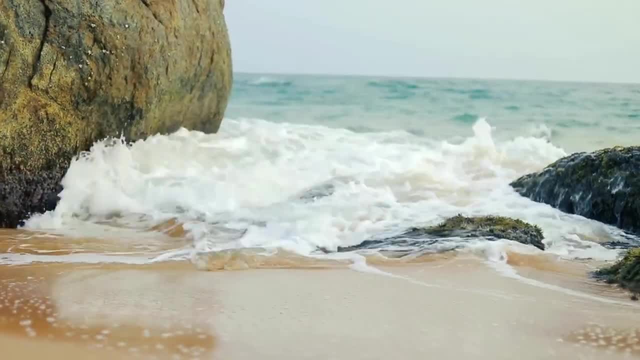 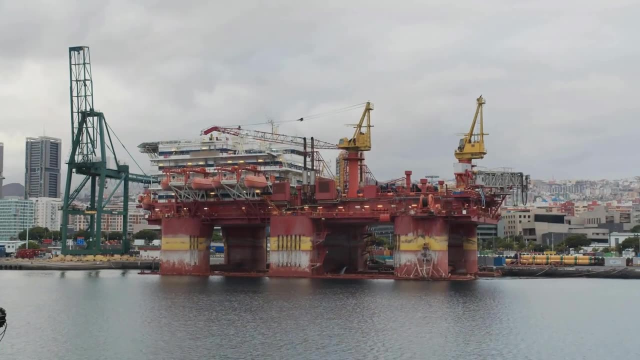 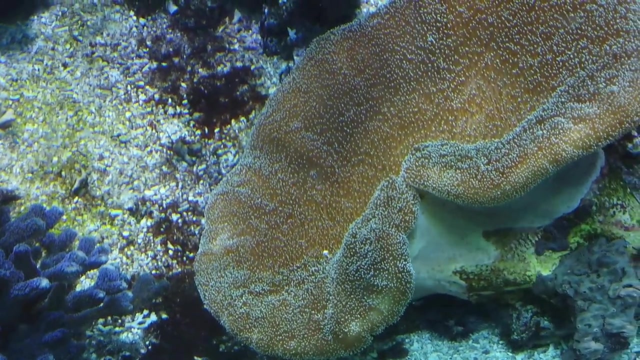 Mining. The oceans, as I mentioned before, are also a source of natural resources, such as crude oil, gold, copper, etc. Thus, ocean mining is inevitable. However, the process of mining for these resources gives room for pollutants to find their way into the marine ecosystem. 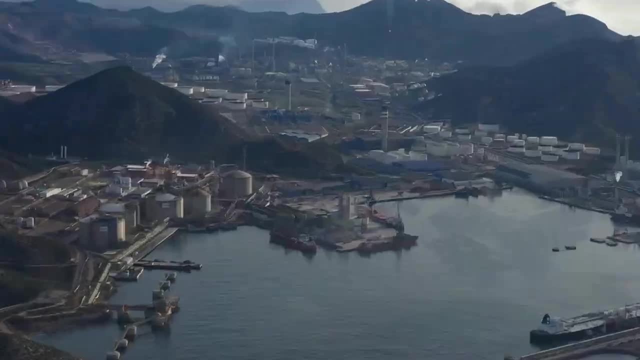 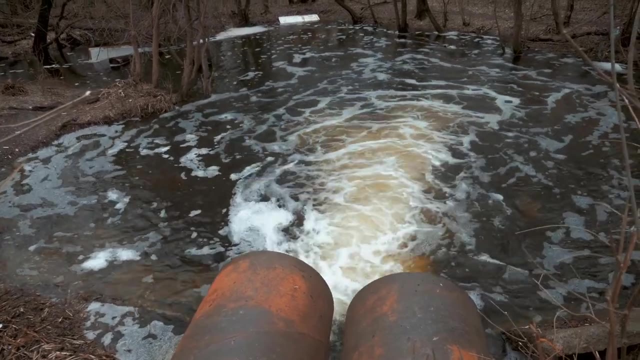 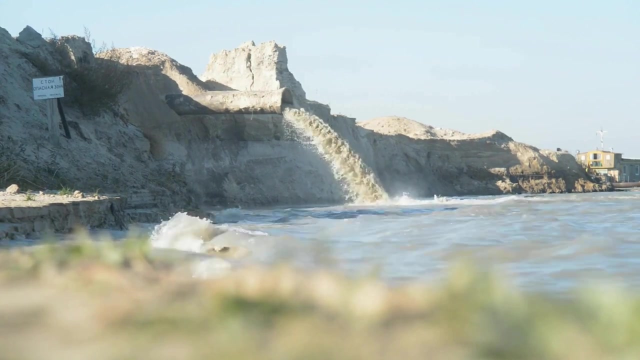 Chemicals from the spills and sulfide deposits deep down the ocean lead to the death of many sea creatures. Sewage: Over the years, dumping of sewage in surface waters has caused several deaths in the marine ecosystem, Whether it gets there directly, as seen when people dispose of wastes in surface waters.